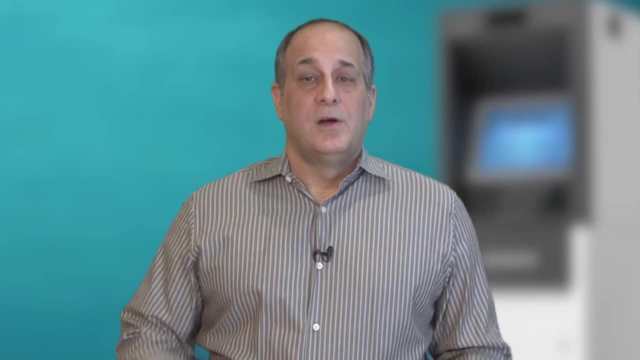 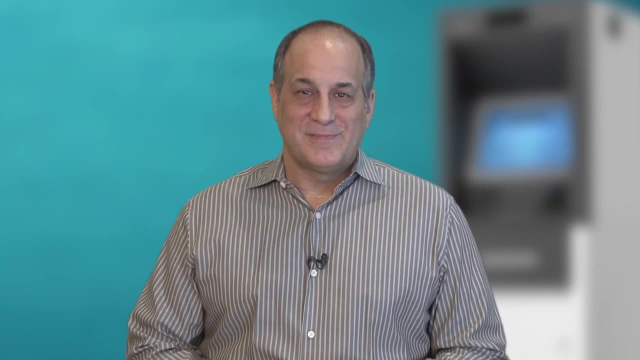 Still All right. All right, I guess we're done. I guess we're done. Okay. so maybe it's not so easy, but eventually there were ATMs that took our card and accepted deposits. The next ATM I tried was a drive-thru. 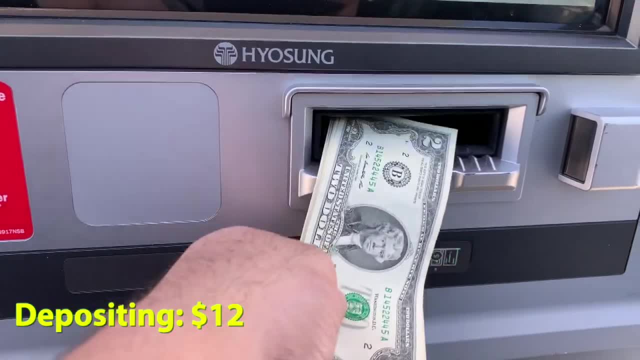 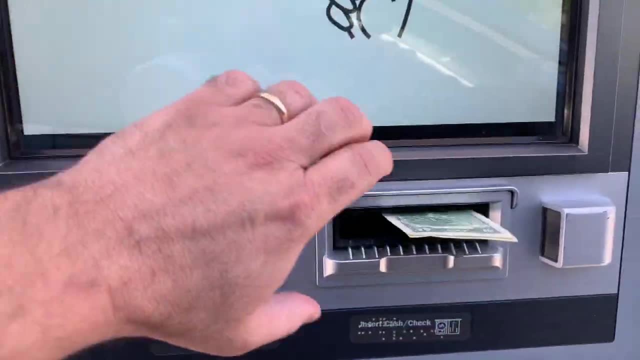 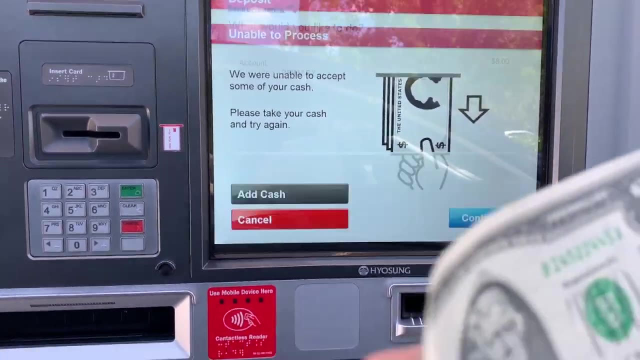 where I wanted to deposit six, two dollar bills. Twelve dollars, All right, Uh-oh. Unable to accept some of the cash, It only gave me two of them back and it took eight dollars. These are the ones it didn't take. 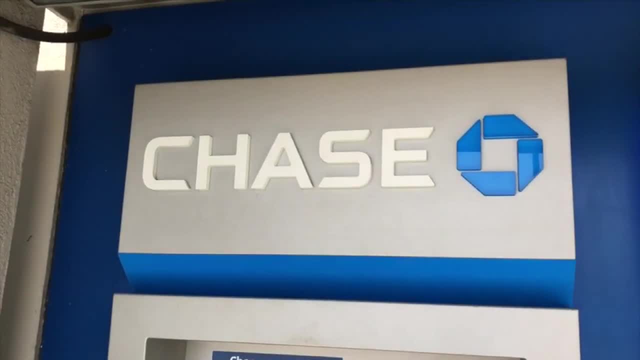 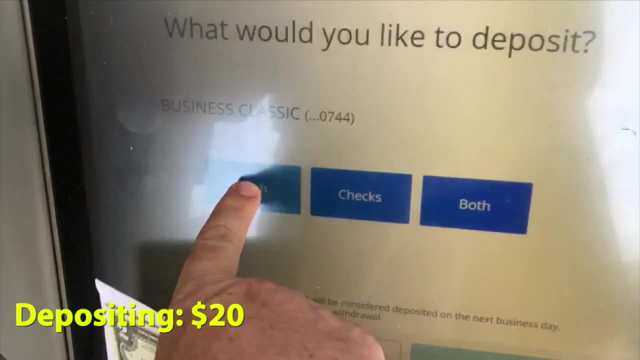 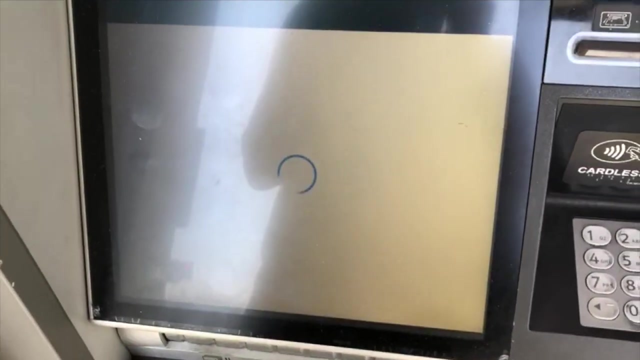 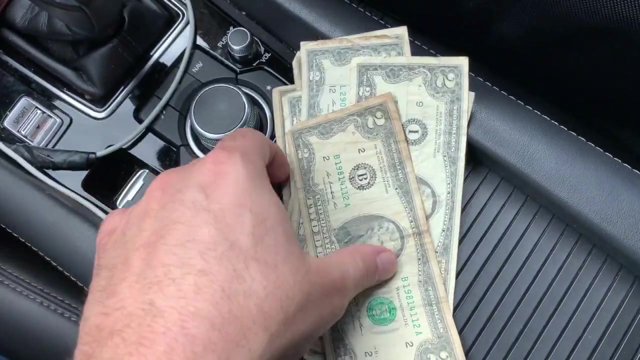 All right, so we'll deposit eight dollars instead of twelve. Chase Bank: We have ten, two dollar bills, so a twenty dollar deposit Cash. There we go Processing. Oh look at that Bam, And it took it. Okay, now we're going to try depositing twenty dollars, and these two dollar bills are very ratty. 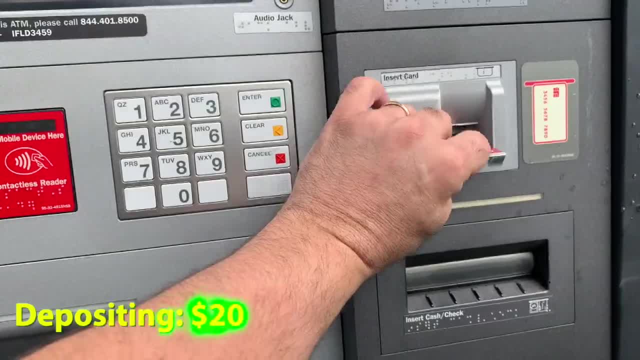 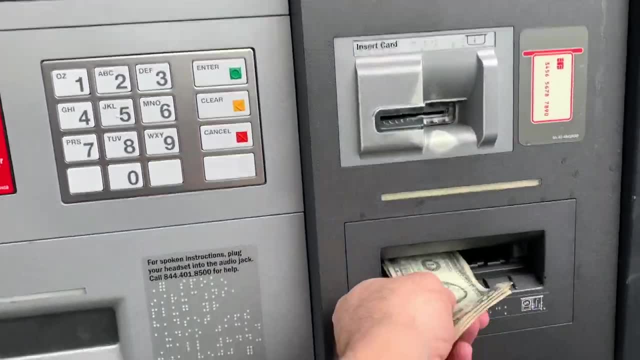 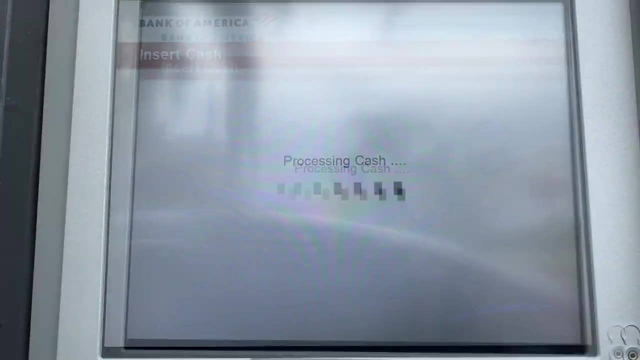 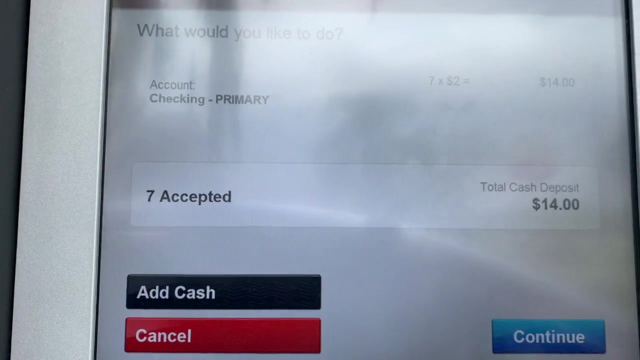 So let's take a look and see what happens. Okay, here they go: Twenty dollars in two dollar bills. Ten of them. Some came back. They were unable to accept some of my cash- Three of them- So they did accept seven out of ten. We'll deposit those. 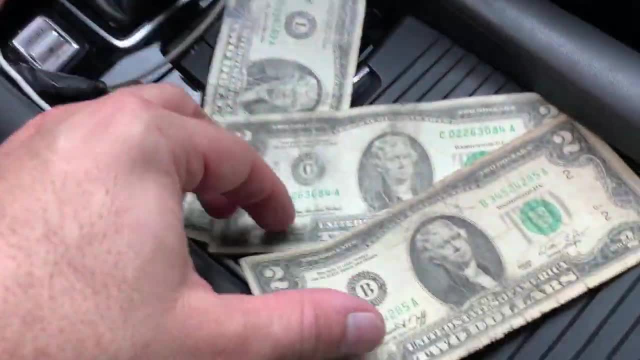 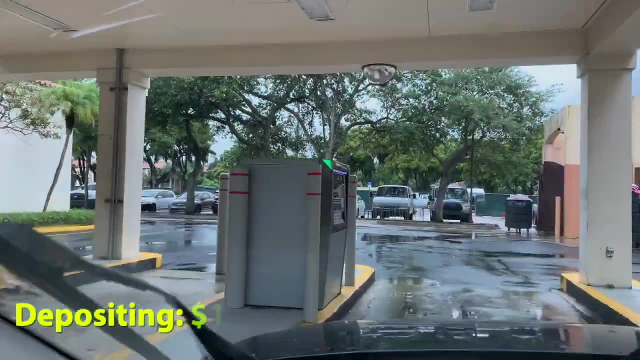 These are the bills it did not accept: One with tape on it and two pretty poor condition bills. But seven out of ten at that ATM. Okay, let's try this bank. We're going to try to deposit ten dollars in two dollar bills. 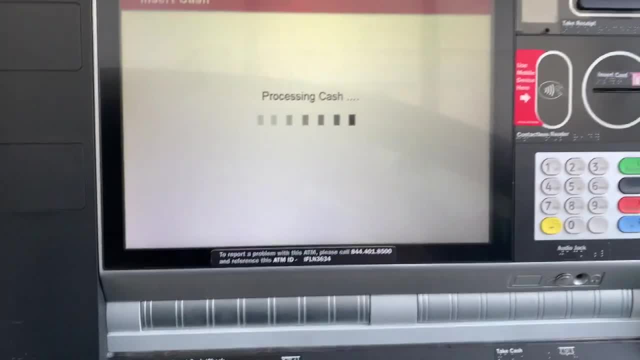 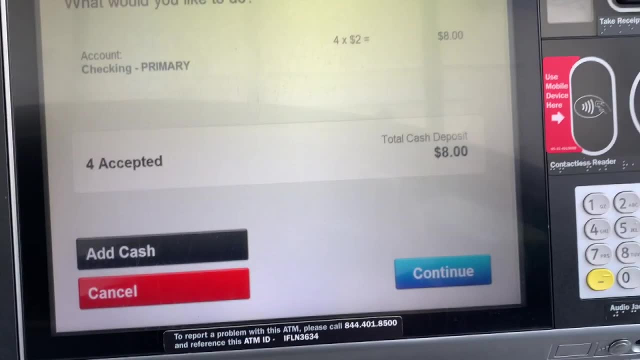 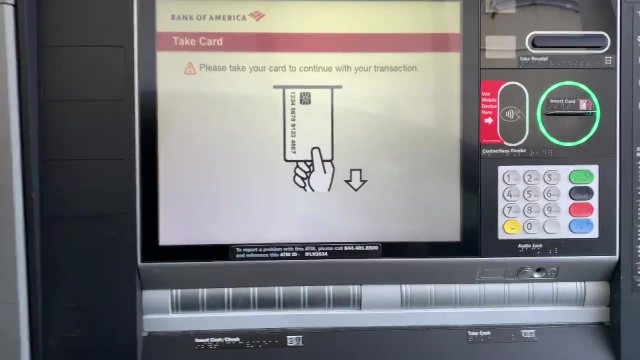 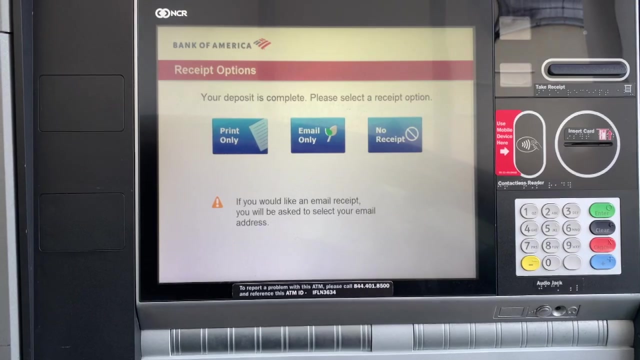 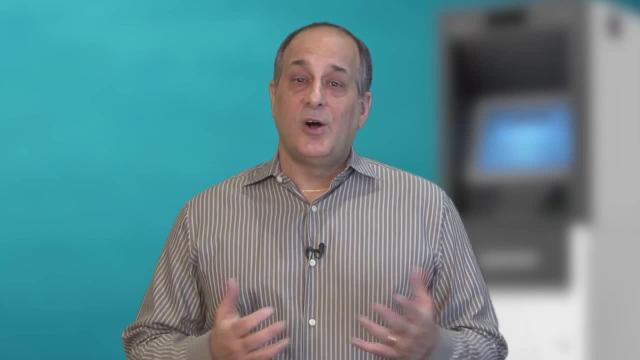 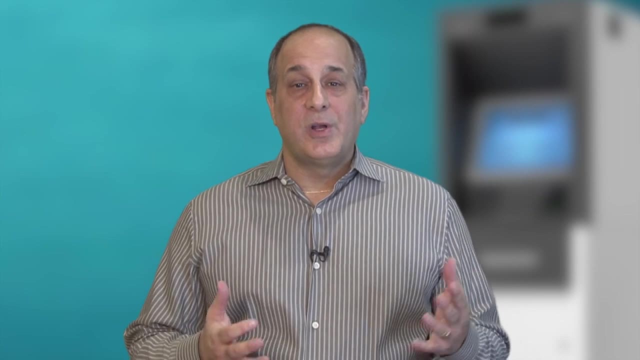 which is that ATMs do take two dollar bills, just not all of them all the time. Frankly, I don't know why anyone would ever want to deposit a two dollar bill. If you're going to do anything with them at all, you should spend them. 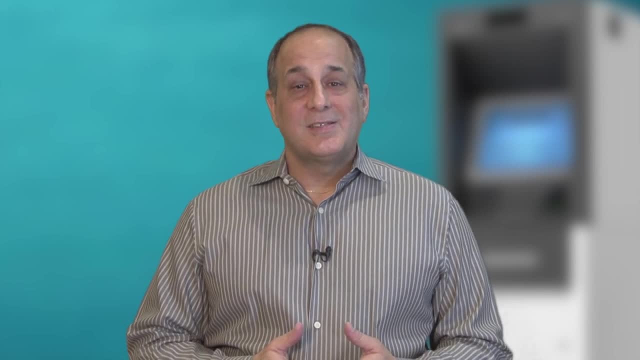 Why? Because of all the benefits you get from doing so, I cited seven of them in this video, Which you should spend four minutes watching right now. Thanks for tuning in. 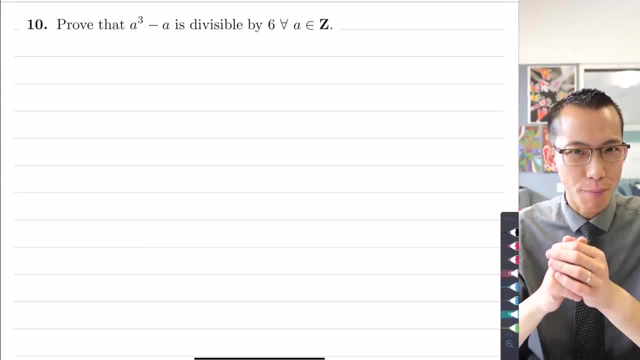 We're going to have a look at this question that comes under the nature of proof, So read it with me and let's think about a couple of approaches we could use to prove this result. Prove that a cubed minus a is divisible by six for all values of a, such that a is an integer. Okay. 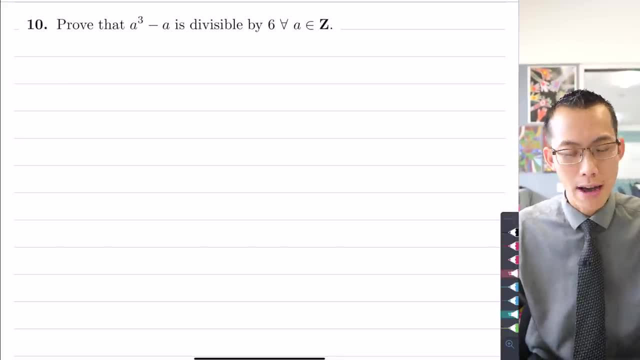 how do we go about this? Now, one of the first things that might come to your mind when you look at a question like this is whether a tool like mathematical induction might be useful here. Now we can use mathematical induction to prove this result, and you can think: all right if I don't. 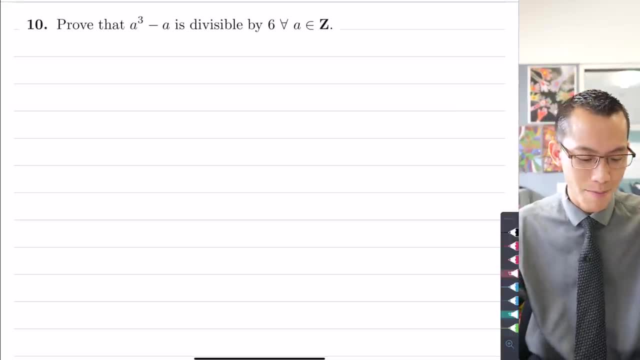 need any kind of- you know, sophisticated knowledge beyond extension one. I might as well just go with that right. But there is a reason why- in fact a couple of reasons at least- why using mathematical induction to prove this particular result is less than ideal. So I'm going to walk you through what. 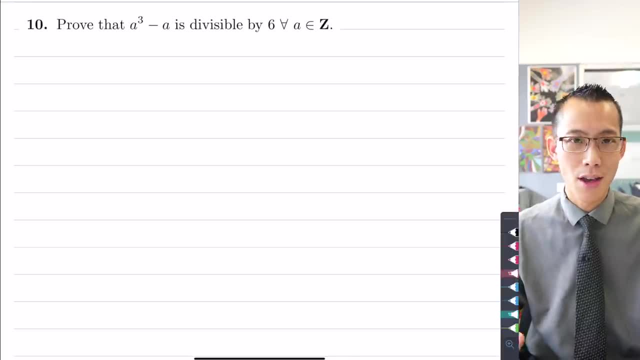 those reasons are, and then I'm going to show you an alternative path for actually proving this result that doesn't rely on induction at all. So let's have a think about how I would lay this out in a mathematical induction. So let's have a think about how I would lay this out in a mathematical 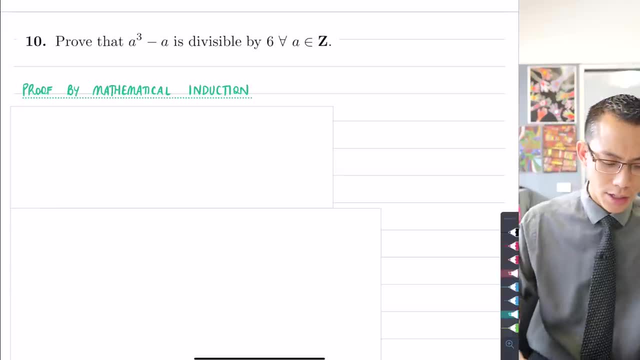 if I were to do this by induction. What's the first step when you begin any proof by mathematical induction? And the answer is: you need to test the base case, the first place, the first value where this statement is true. Now, this is where you run into your first snag, because when you